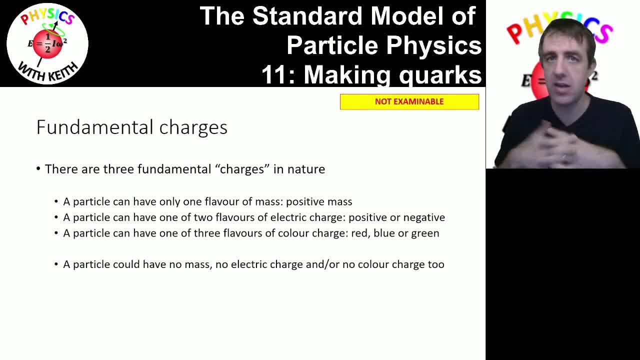 all mass is attractive. There's only positive mass. we've never detected any evidence of negative values. Thanks for watching. never detected any evidence of negative values mass, Whereas electric charge has two flavours, positive and negative, and the interaction is interesting. Like charges repel, unlike charges attract, and we can use Coulomb's law If you. 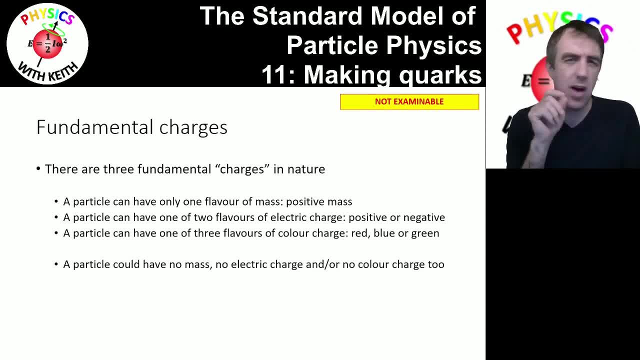 remember, right back at the beginning of this series I said the graph for the strong nuclear force was much more complicated, and it is The strong nuclear force acts between particles that have a different sort of charge, which Murray Gell-Mann called colour charge, And he only called. 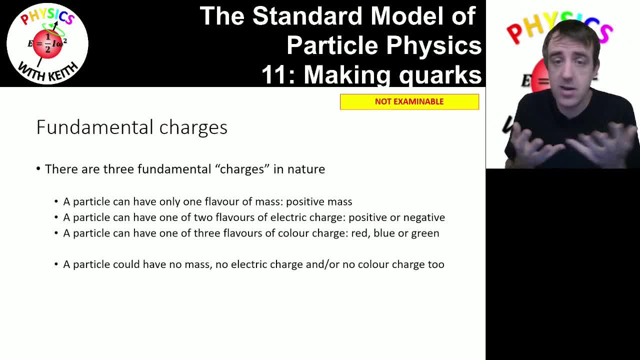 it colour charge, because we needed another way of identifying with this type of charge. And, unlike gravity, which has one flavour, an electric charge that has two flavours, this type of charge has three flavours. Oh, and three anti-flavours: Red, blue and green is how. 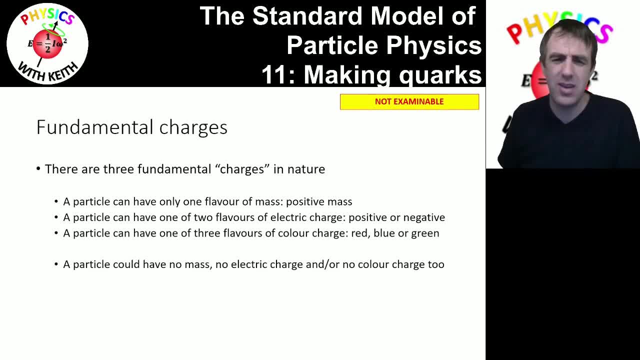 we name them by convention. But don't confuse this into thinking the particles actually have those different colours. They're just a way of labelling this colour charge that the particles can have, And so particles can have a selection of these different charges. You can have particles. 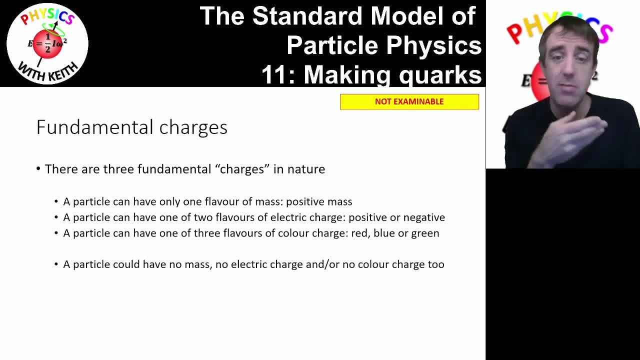 with no charge but they have got mass. Or you can have particles with mass and with charge. You can have particles with colour charge and electric charge and mass, So you can get a selection of all of these. There are four fundamental forces in nature that relate. 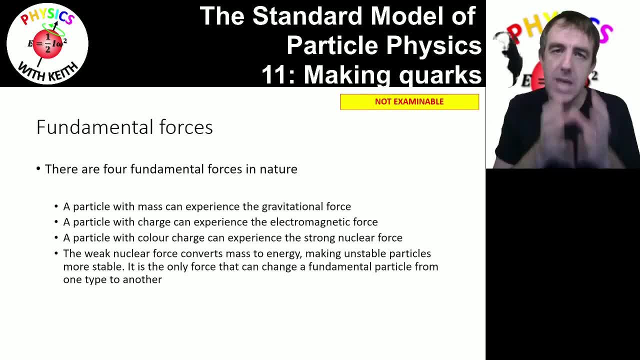 these three fundamental charges: Mass experiences the gravitational force, Charge experiences the electromagnetic force, And it's colour charge that experiences this strong nuclear force. So only quarks have colour charge. Leptons don't have colour charge. And then of course there's the fourth force. 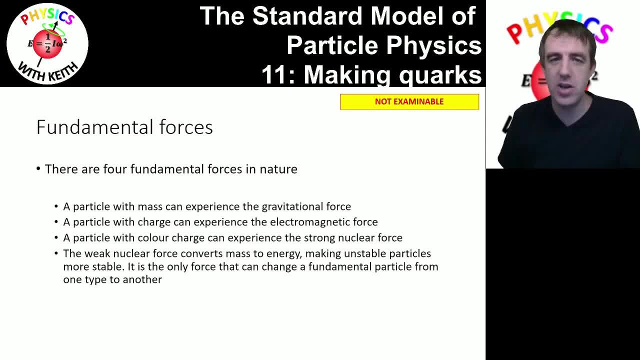 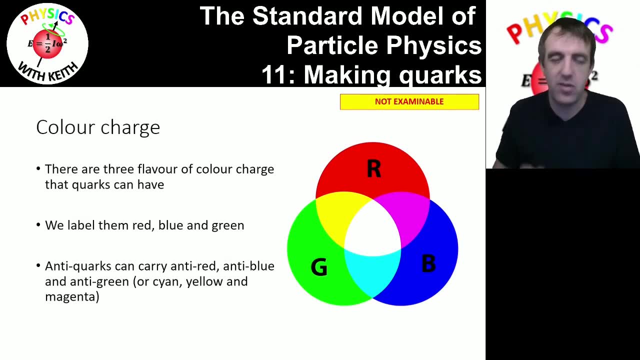 fundamental force there, turning mass into energy and vice versa, rather than producing a measurable acceleration on particles or something Like that which we might naturally think of as a force. So why did Murray Gell-Mann pick colour as a model for this new type of charge? 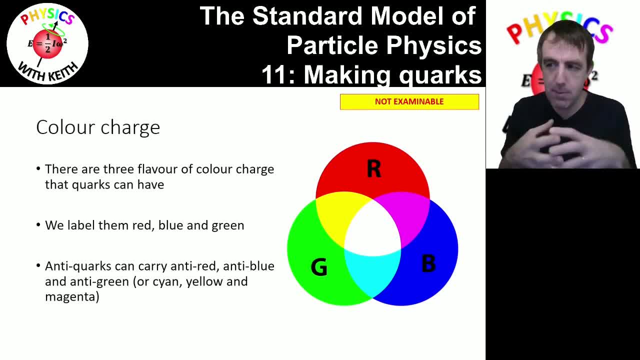 Well, it's because of the fact that you get three quarks combining to form a baryon. The idea is that particles have to be colour neutral. That means that a quark has to contain a red, a blue and a green colour quark in order to have the overall colour of the baryon. as 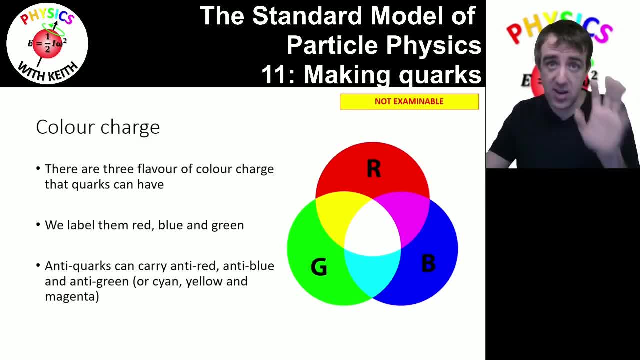 white, So it's colour neutral. Anti-quarks carry the anti-colours, So anti-green sometimes called magenta, anti-red sometimes called cyan and anti-blue sometimes called yellow, And so anti-quarks carrying those three colours can combine to form an anti-baryon. 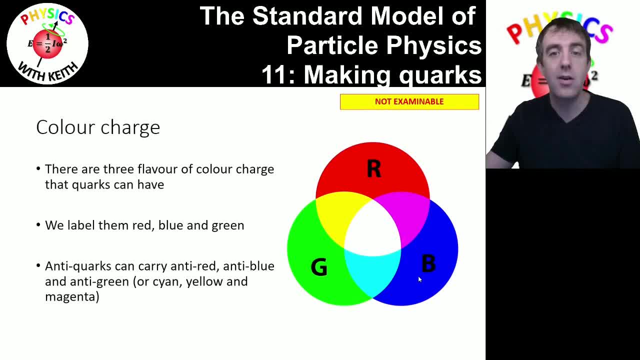 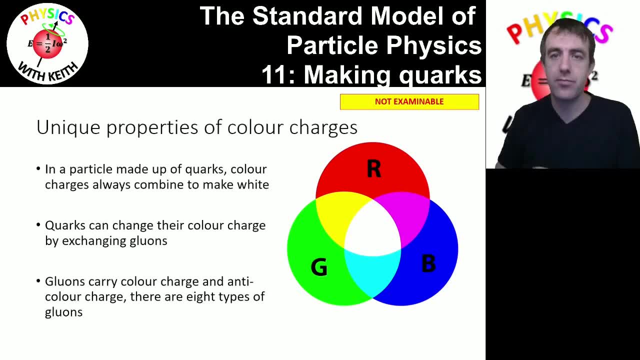 Because anti-red, anti-blue, anti-green or cyan, magenta and yellow, when mixed together, form white, So colour neutral. Now, this model's built up on the observation that there are always three quarks or three anti-quarks in a baryon or anti-baryon. That's what makes this model come together. 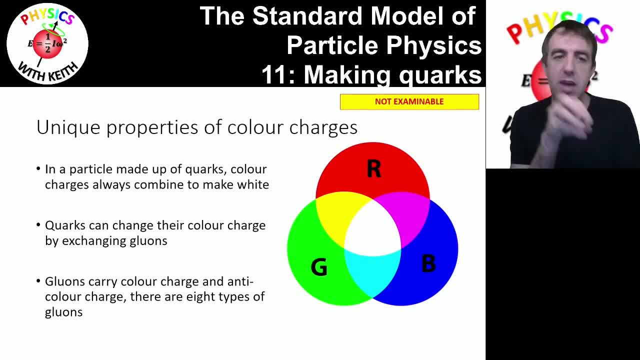 What's fascinating is that quarks don't have a fixed colour charge. They change their colour charge, And that's what gluons do. When a gluon is exchanged from one quark to another, it carries with it the colour charge and swaps them around. 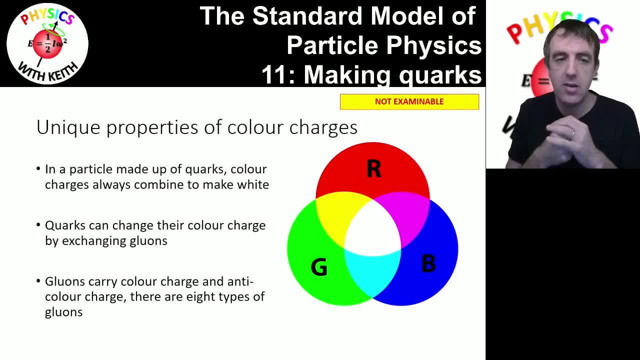 It's constantly changing. It's constantly changing the colour charge of these quarks. This subject is called quantum chromodynamics: Quantum, because the colours can only have certain values, Chromo referring to colour and dynamics, the idea that these are changing. But again, the world's not quite done. 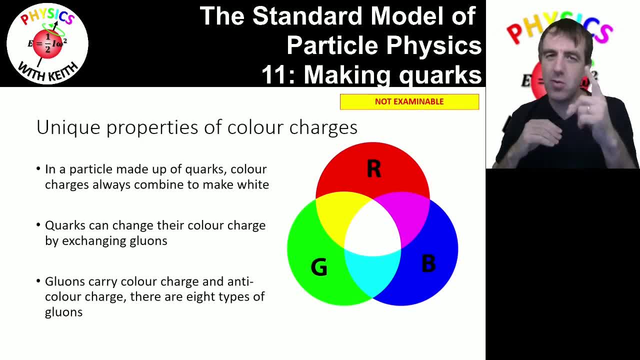 with being fascinating. yet Gluons don't just carry one colour charge, They carry two. They carry a colour charge and an anti-colour charge. Gluons have two different colour charges: A colour charge and an anti-colour charge. Quarks have. 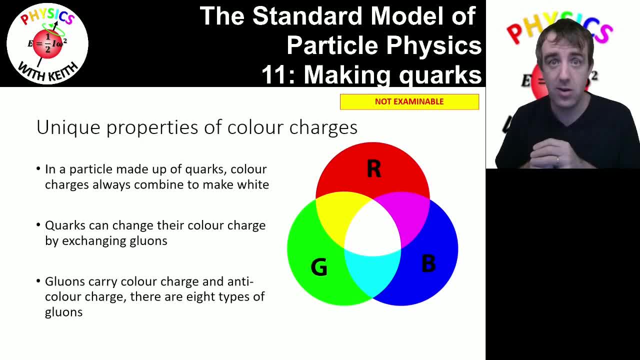 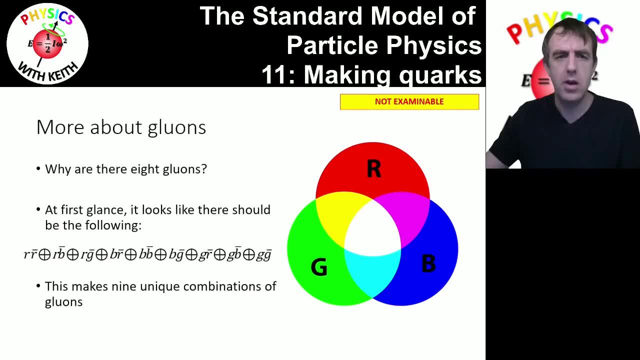 either a colour charge or, if they're anti-quarks, an anti-colour charge. Gluons have both And you can mix and match. So that's why it seems a bit odd that there are eight types of gluon. So on the face of it it looks like there should be nine types of gluon. You could have a red-anti-red. 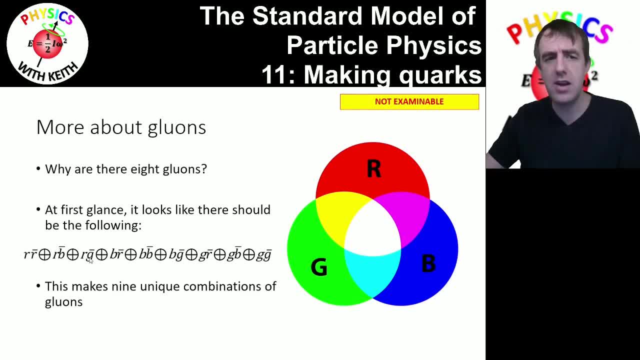 gluon, a red-anti-blue gluon, a red-anti-green gluon, and then you could have a blue-anti-red gluon, a blue-anti-blue gluon, a blue-anti-green gluon, and then you could have a blue-anti-red. 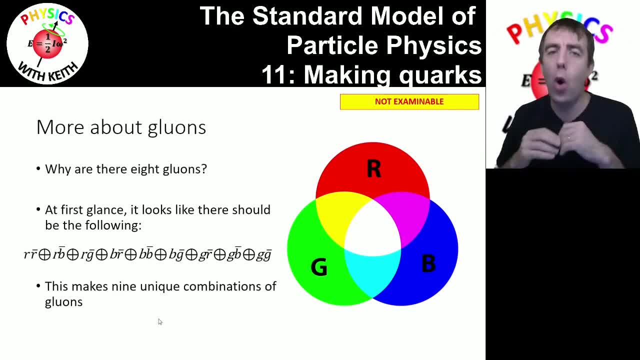 green gluon and so on, This symbol in the middle means or in statistics, So you could have this type of gluon or this type of gluon or this type. And in probability, when you multiply probabilities together, you are saying: and So this string here is the probability of this. 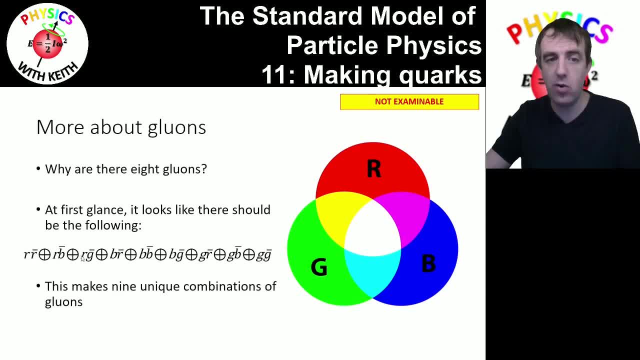 and this or this and this or this and this or this and this, And one of the ways you can write that is using a plus and then using some normalizing factor to make the probability back to one. You've done probability probably further down in your schooling where you may have learned. 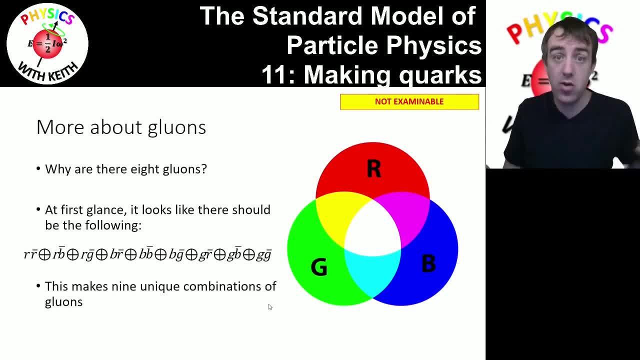 that when you say the probability of one thing and another, you multiply the probabilities, but the probability of one thing or the other, you add them together. And so if I have a gluon, it has a probability sat with this equation where these are pluses, these circles with pluses. 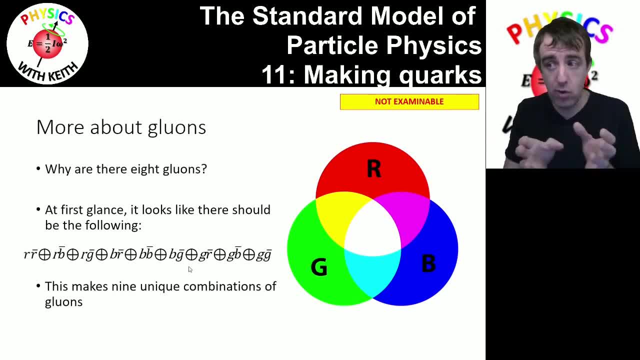 in them they're multiplied by some factor that makes the overall probability one. That looks quite nice, but it's not quite right, because that's nine combinations and I've just said there are eight combinations. Well, let's see if we can knock some of these out with some basic classical. 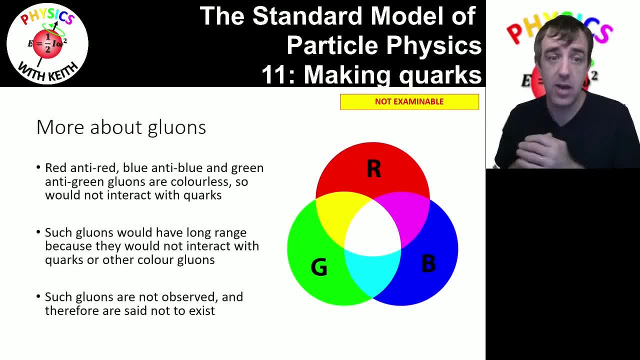 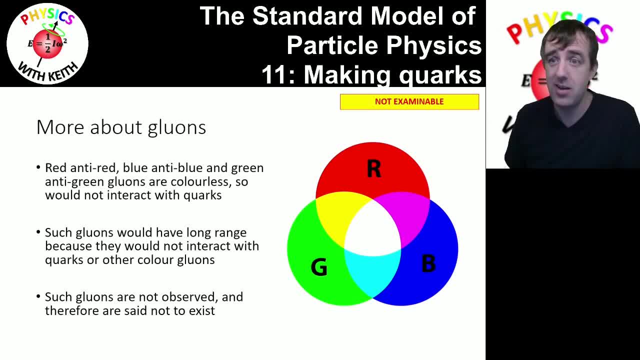 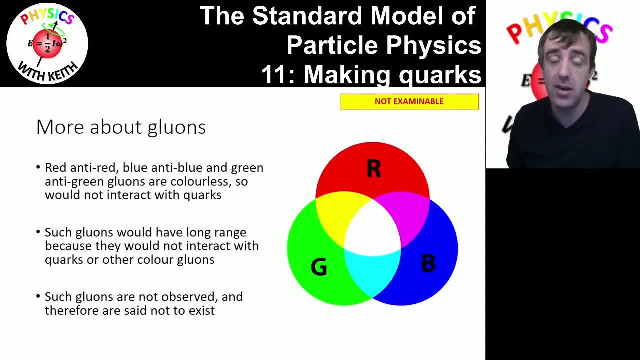 why say it exists at all. We're going to employ Occam's razor. Occam's razor is the idea that if we've got a model that works and there's another model that works that's simpler, use the simpler model. There's no point having a more elaborate model if it predicts the same. 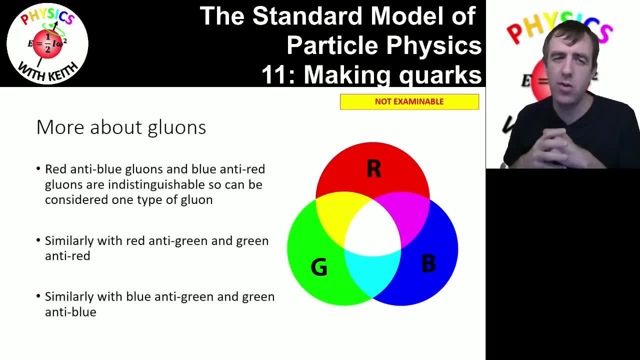 results. There's also an idea here that red-anti-blue gluons would interact with red quarks and blue quarks. Well, so did blue-anti-red gluons, So they would be indistinguishable from each other. So we can start bunching together some of these gluons and saying: 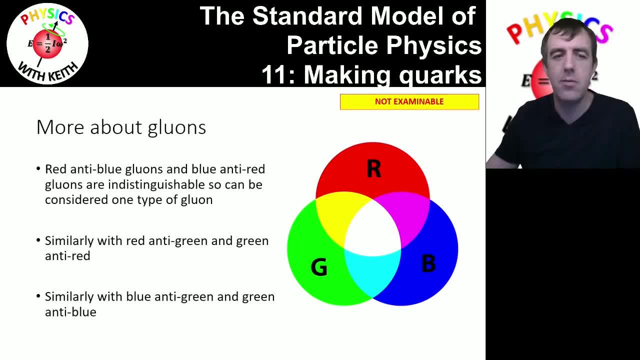 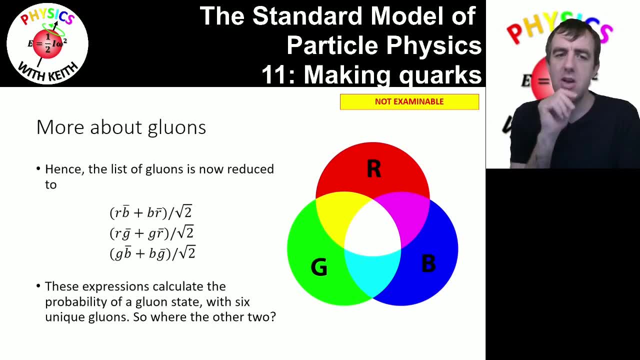 well, they're indistinguishable. Let's just say they're one type of gluon, And we can do the same thing with red-anti-green, green-anti-red, and with blue-anti-green, green-anti-blue. When you do that, you end up with three gluons. Oh, hang on. I said there were eight. 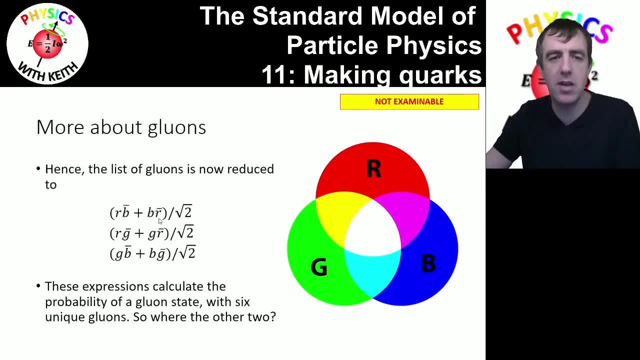 I've gone too far the other way. now, Again, this is a probability expression. So this is red and anti-blue, or blue and anti-red, and then multiplied by some factor to normalize that probability back to one. So where are the others? 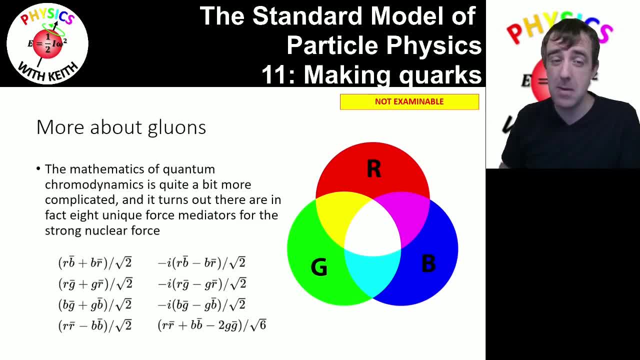 Well, I'm going to show this list and I'm not going to explain it because I don't understand it. See, it turns out our classical physics way of looking at things- little particles bouncing around and interacting with each other- is severely limited. 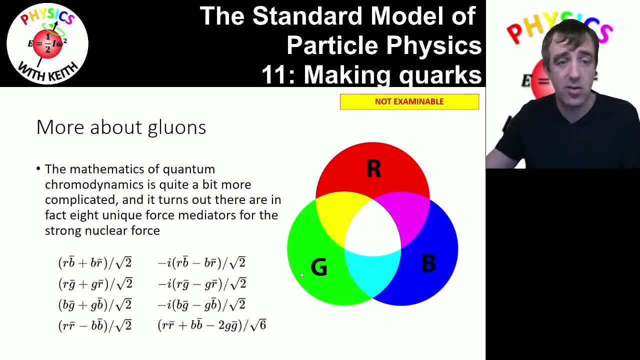 That's not the way the universe really is. These particles and all the other particles that you've seen in the particle zoo, those symbols, are wave functions. They are functions that tell you the probability of a particle, the probability of its energy, the probability of its 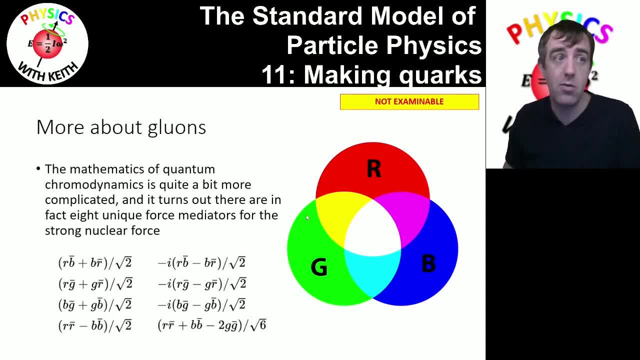 momentum, the probability of the particle- How likely is it to be where you think it is and to be what you think it is? That's all tied into those wave functions, And wave functions can interact with other wave functions, And that's what you're looking at. here is eight unique operators that will be used to transform. 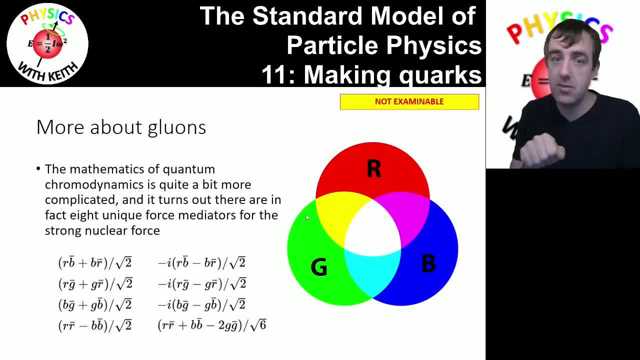 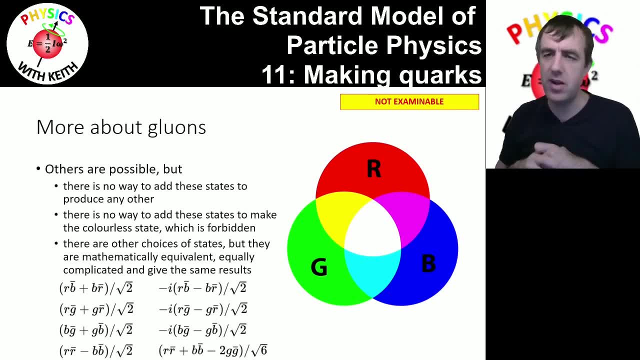 one set of wave functions to another set Incredibly complicated and sophisticated mathematics. When you look at these you think what does the i represent? That's the square root of a negative number, square root of negative one. So you've got imaginary things here. 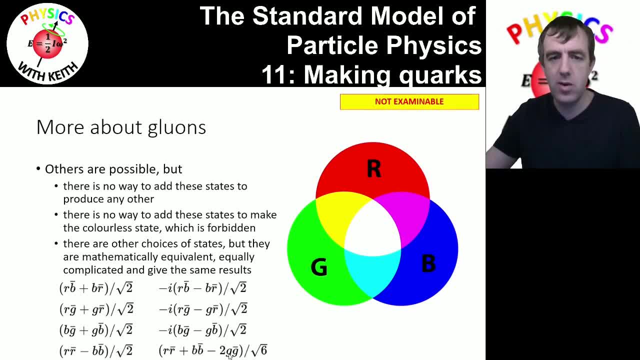 If you look at the last one on this list- red anti-red, blue anti-red, blue minus two green anti-green- Well, is there a blue anti-blue, red anti-red minus two anti-green, two green anti-green? Well, yes, but it does the same thing. So there's all sorts of 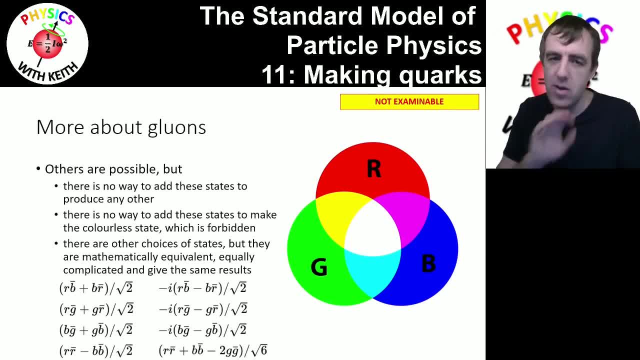 other ways of writing these gluons, but you don't need to, So we're going to use Occam's razor. The minimum number we need for all of our strong interactions is these eight, But there are other formulations of this. We just don't need them Now. I know this is complicated. It is complicated. 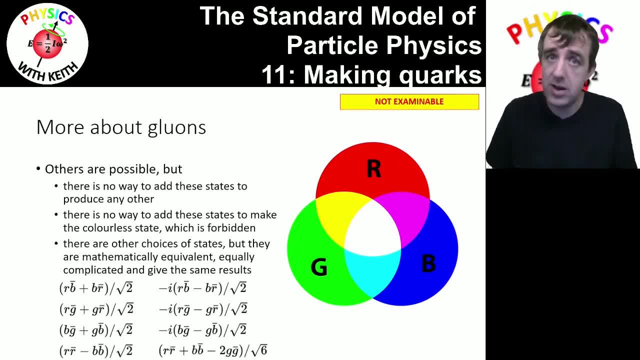 That's why part of this is complicated. Particle physics is famously a difficult subject And we desperately want to try to visualize it in terms of lumps of matter moving around Classical physics analogies that we try to use. just they don't work for particle physics, which is a real shame, because it'd be lovely if they did. 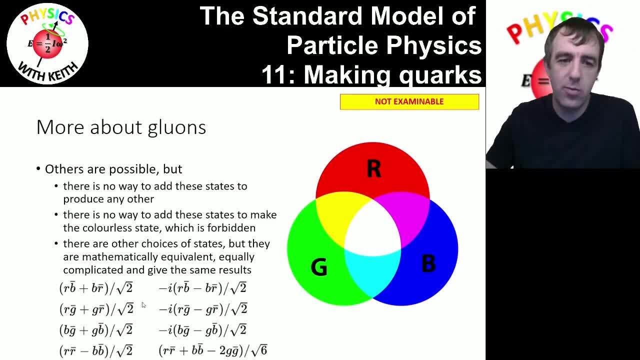 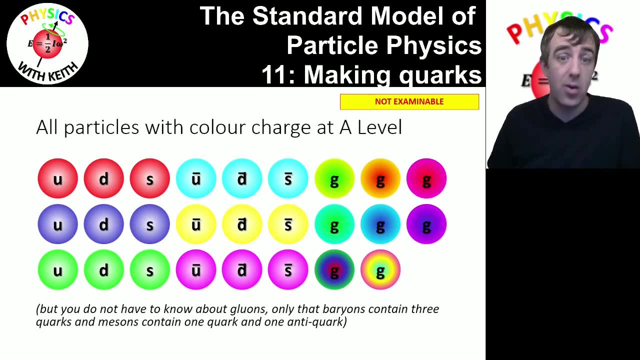 So instead we have to use complicated things like this. These are wave functions that you use to transform one wave function into another wave, So we're going to use the wave function. Okay, If we did want to have some sort of visual representation of these quarks and gluons, then for A-level, this is what it looks like. Notice I? 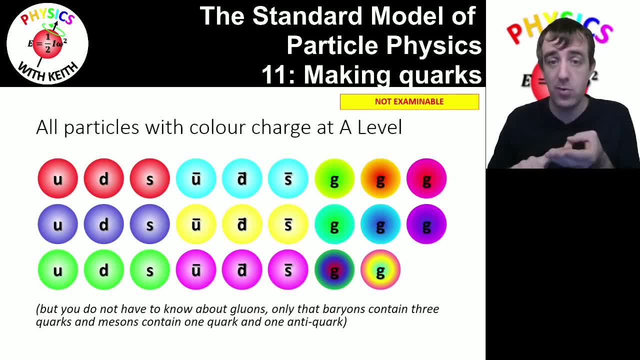 haven't included the charm quark, the top quark or the bottom quark here, But I have included the three different colors of up, the three different colors of down, the three different colors of strange, the three different colors of anti-up, anti-down, anti-strange and all eight gluons. 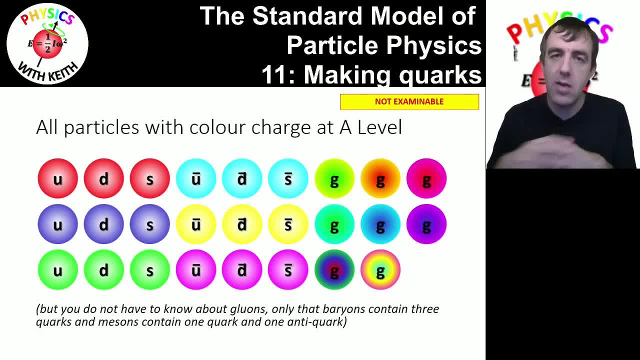 Whatever that is, They are, It looks like quite a lot. Again. we will have this really lovely picture with quarks, and we managed to get that list of fundamental elements that the universe was made out of into a smaller number, And now we've just increased it again, And we have increased it again. 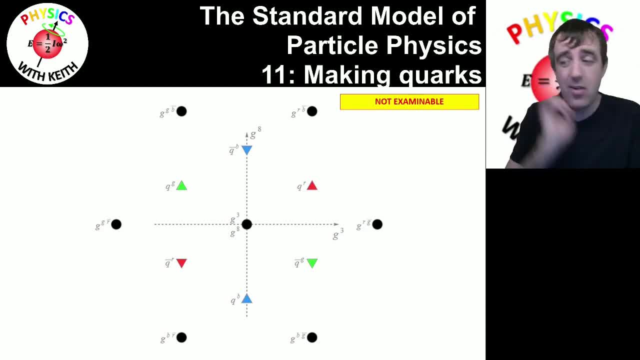 but it's not too much. You can find diagrams like this that are supposed to help you see which gluons are exchanged between which quarks. So a red quark here and a green quark here. there are certain gluons that can be exchanged between them. 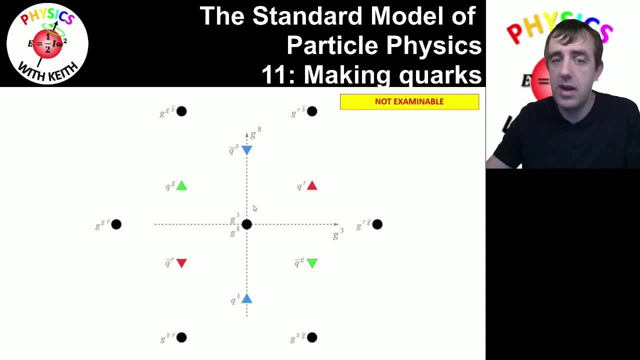 This gluon here, G3, whatever that is, But this quark here and this quark here. they can be. the interaction between those two quarks can be this gluon or this gluon. Now you'll find particle physicists love diagrams like this because it helps them. 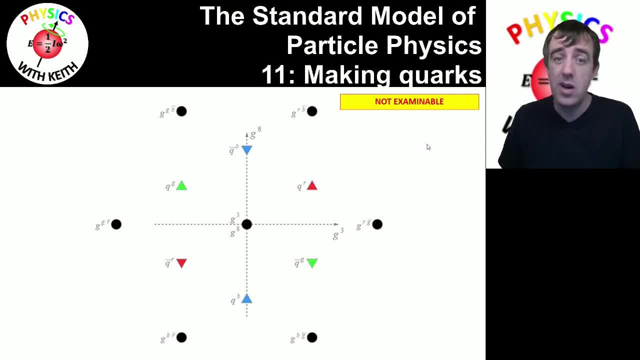 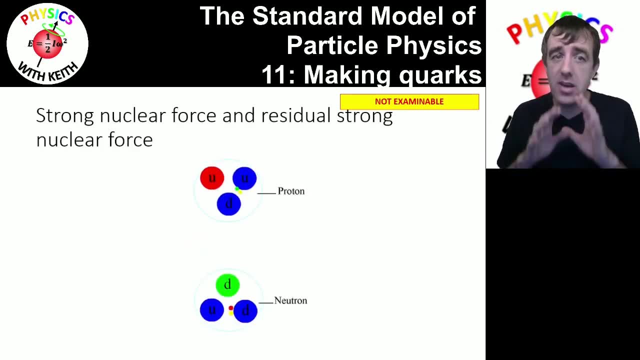 understand what's going on, But if you don't really know what the gluons mean, then they're not actually much help. So let's try for a nice, easy classical physics model of what's going on. If you look here, you can see that within each of these baryons this is a proton. this baryon. 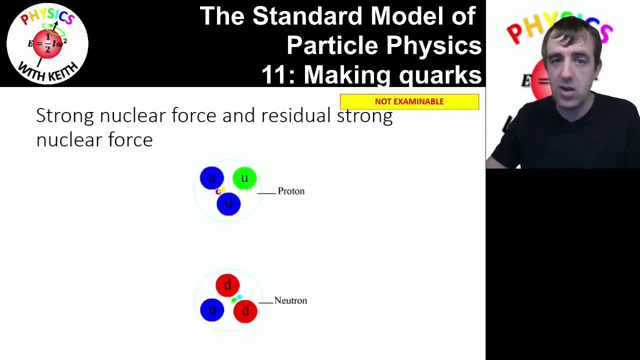 there are gluons being exchanged. The gluons carry a charge and an anti-charge. When those gluons are exchanged they switch around the colour charge of those quarks, But overall the quark remains white. It still has red, blue and green inside it. 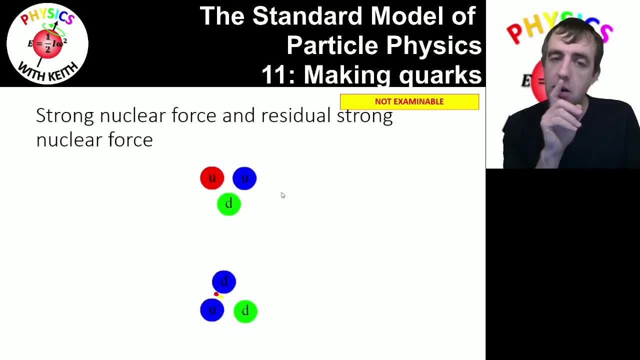 Now those gluons cannot go very far. They can't go very far because they exchange gluons with other gluons, But the gluons can decay into quarks and anti-quarks in equal number. Now those quarks and anti-quarks which form a pion can't go very far either, because they 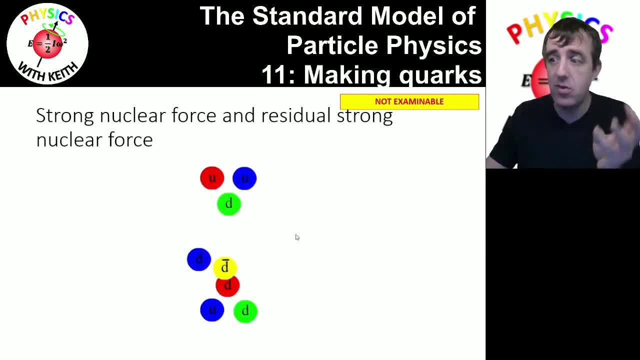 will eventually annihilate. They're in a metastable state. They exist for a small amount of time, long enough for them to leak out of the baryon and bridge that gap from one baryon to the next. So Yukawa said that pions were responsible for the strong nuclear force, And he's not entirely. 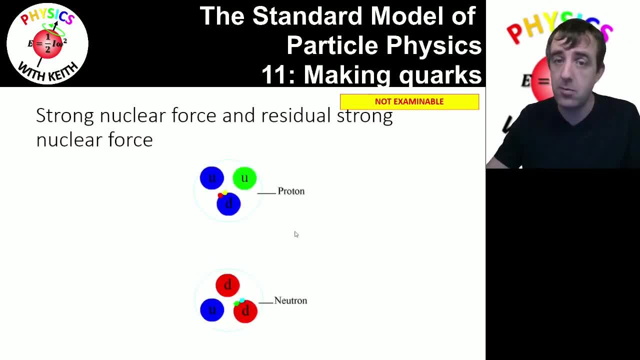 wrong. They're responsible for the residual strong nuclear force. That's the force, the strong nuclear force that leaks out of baryons and the reason why baryons bond together within the nucleus Yukawa was trying to describe. Yukawa didn't have a quark model, So he was trying to explain. 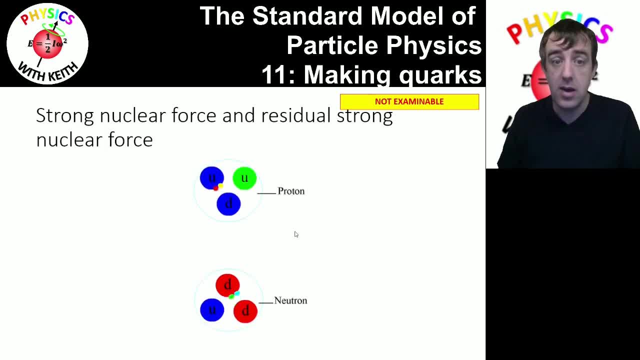 why protons and neutrons stick to each other in the nucleus, And actually pions give you that explanation. They act as a conduit, a bridge from one baryon to the other, so that the strong nuclear force can get out of a baryon. What's not shown in this little animation? 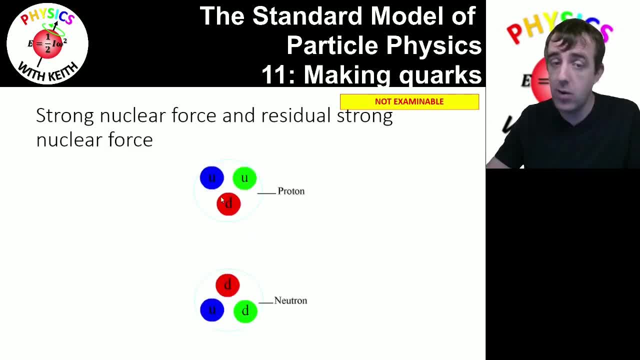 is that you will also get quarks and anti-quarks created in equal measure within the baryon, constantly, constantly in flux. The mass of a proton cannot be pinned down, or a neutron or any other baryon. You can't pin it down because within that gluon field inside the baryon, 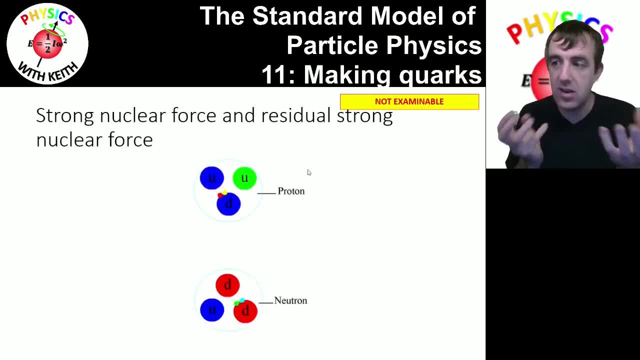 you will always get quarks and anti-quarks being created and annihilating each other, as well as these three quarks. So these three quarks are sometimes referred to as the valence quarks, because they reveal to you what the baryon is. 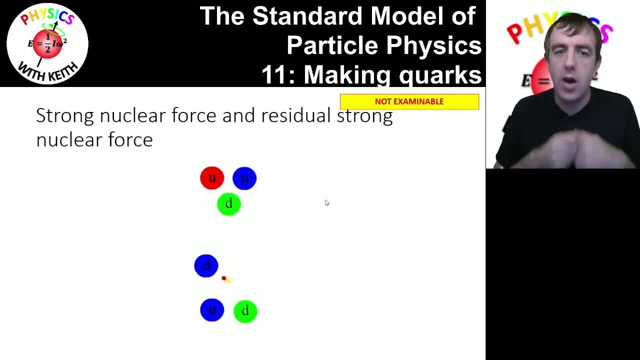 Yukawa said that pions were responsible for the strong nuclear force and bridge that gap from one baryon to the other. They're still a soup of gluons and quarks, being created and destroyed constantly and in doing so, changing the colour of these quarks. So the strong nuclear force is. 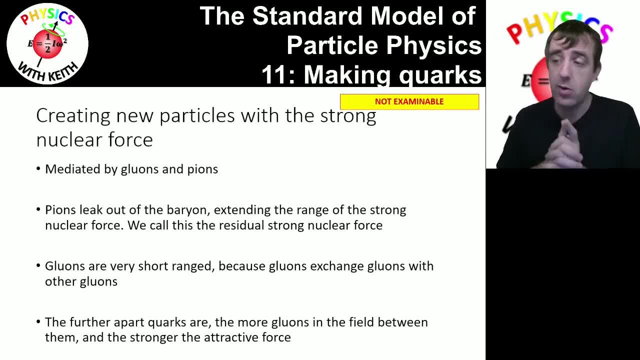 mediated by gluons, but the residual strong nuclear force is mediated by pions. Now the idea that gluons exchange gluons with other gluons can be quite a complicated idea, But what it means is that the further apart you try to get two quarks, the more complicated the idea becomes. 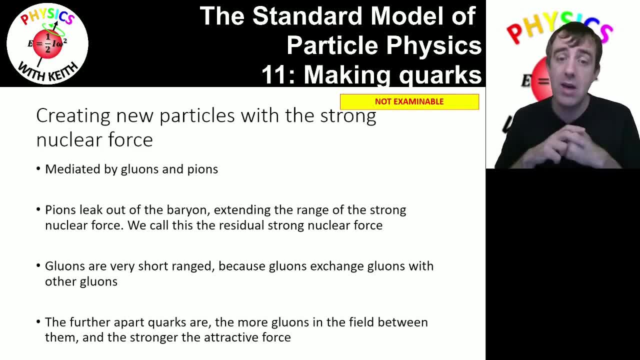 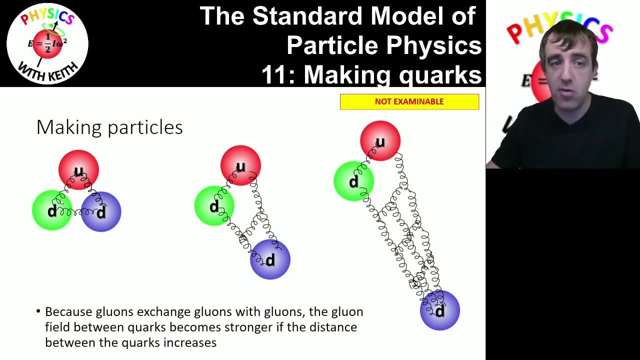 If you have two quarks that are exchanging gluons, the more gluons you'll get between them and these gluons will attract to try to form white, to try to have a colour neutral particle. So if you have a look at this picture, here we've got three gluons indicated with these springs. 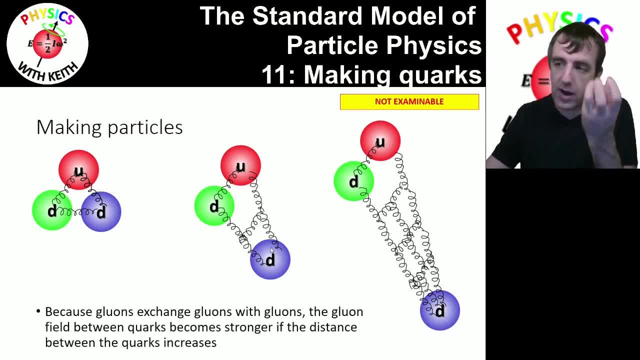 and three quarks. And if I pull the blue quark out a bit then now the gluons here exchange gluons with the gluons here. It's a bit difficult to see. I hope you can see the mouse cursor okay, but the gluon between the green and the blue down quark. 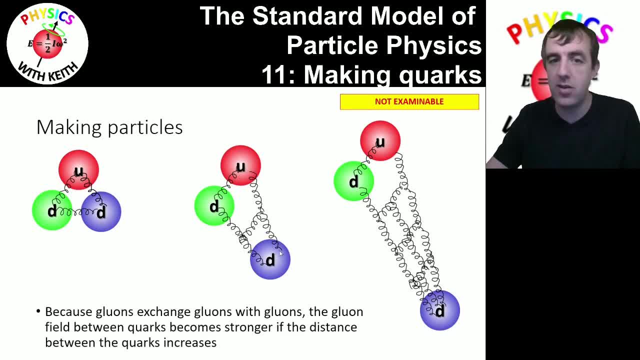 is exchanging a gluon with the gluon between the up and the blue down quark And if I continue to pull that blue quark out then I have more and more gluons being created within this field. The energy, the work that I do in moving that down quark is stored in that gluon field. 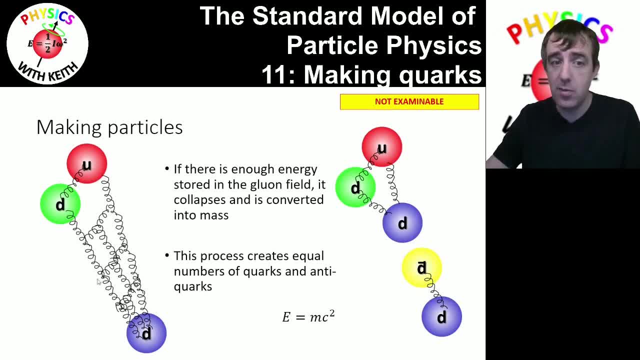 And eventually, if I pull hard enough, then there'll be enough energy, right, There'd be enough energy in that gluon field to create more mass and will create equal quantities of quarks and anti-quarks, in this case, a down and an anti-down. 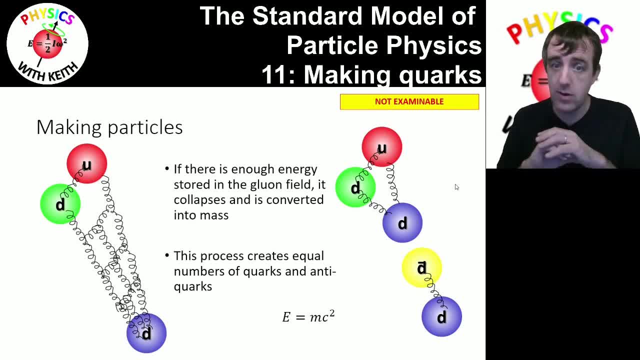 We've created as much matter as antimatter That's allowed. You can do that with the strong nuclear force, And the matter has come from the energy stored in the gluon field. So a question might be: well, how is it that you pull a quark out? You can't.